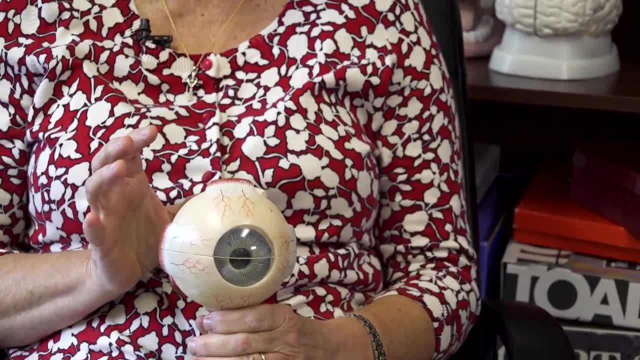 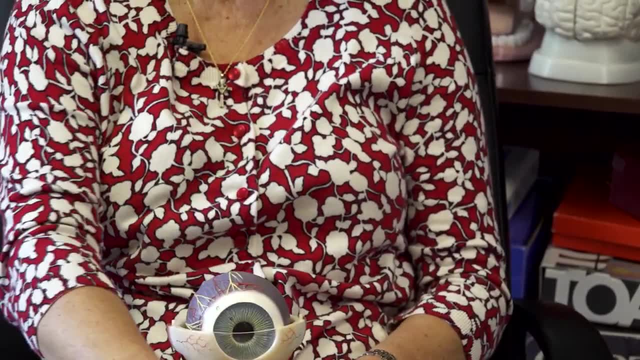 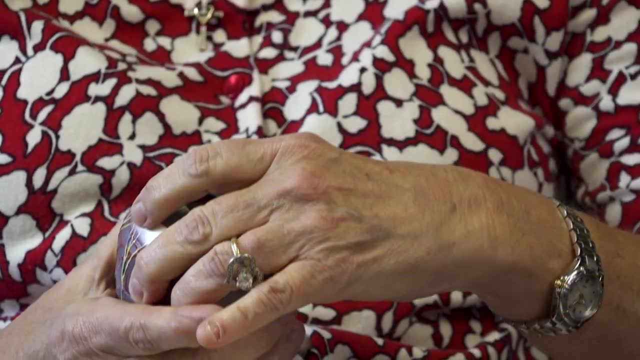 the eye like that. Those are six different muscles and they are controlled by different cranial nerves. Deep inside of the eye, you're going to see another set of muscle which is known as the iris, And then, deep inside, further inside of the eye, there's going to be this muscle right here. 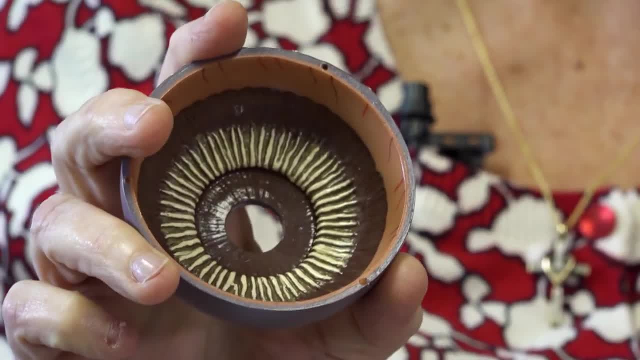 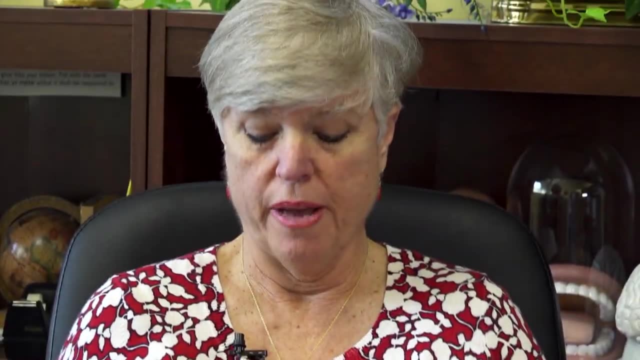 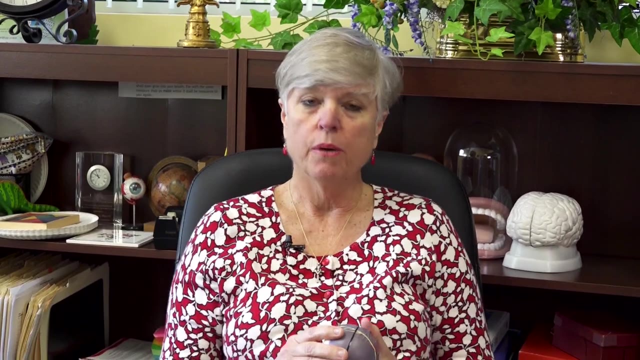 called the ciliary muscle. That muscle affects the shape of the lens And I will say to you- this is what I so often find is weak in children who have visual processing problem. How do I know it's weak? Because they fail a simple test. What happens when a child can't do that? They are going to. 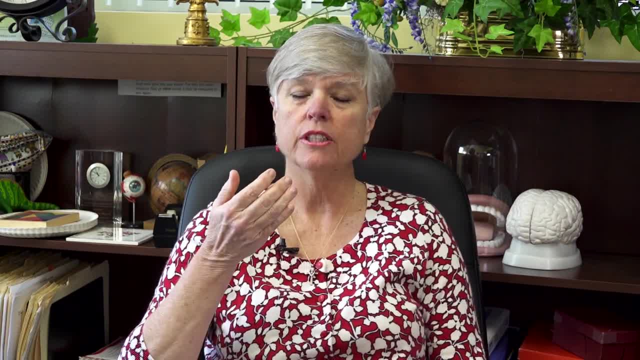 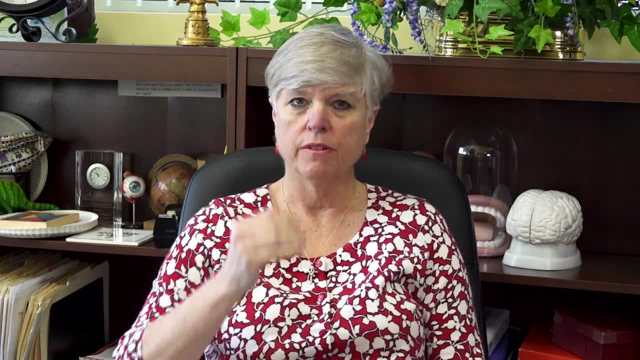 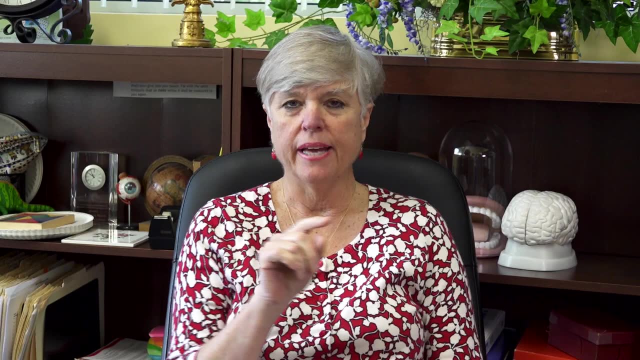 lose focus. And when their teacher is showing them something on the board and then they have to look down the piece of paper, they're going to lose the ability to clearly focus and change focus rapidly. The child, if the muscles are weak, here they go to read something and they're going. 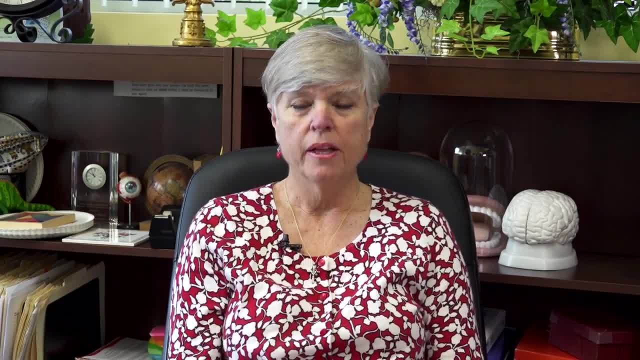 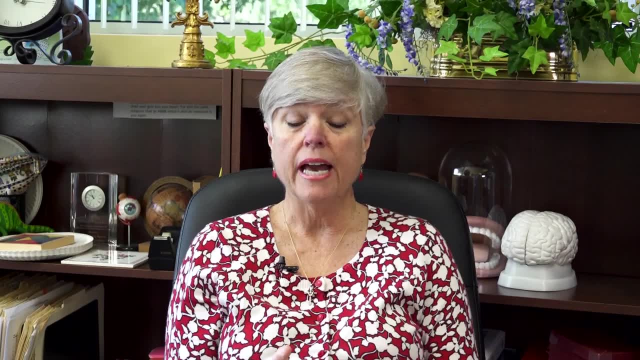 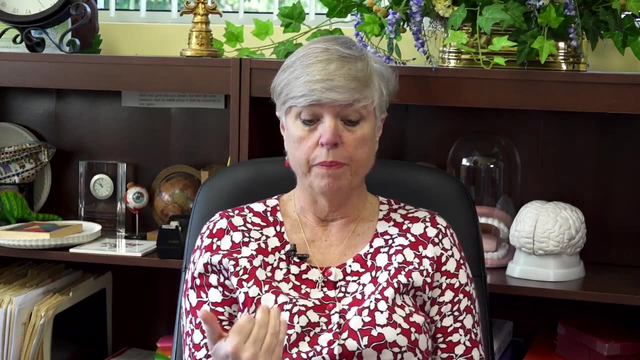 to skip over their words, or they skip to the next line. A child will also. if these muscles are weak, they're going to get confused in looking at numbers, And when they go to read the number 16, they'll read the number 61, or they might even call it 60. And so the visual has such a strong 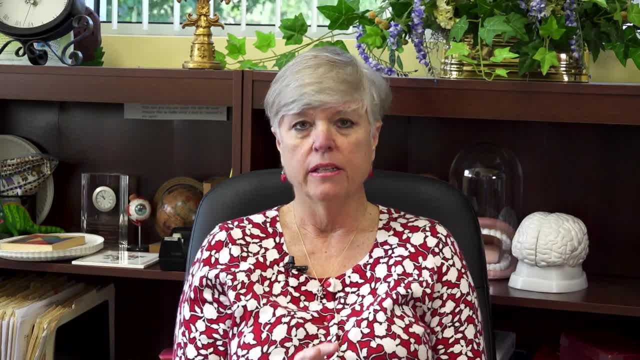 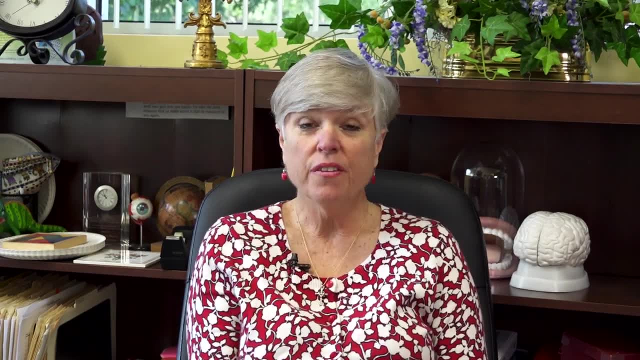 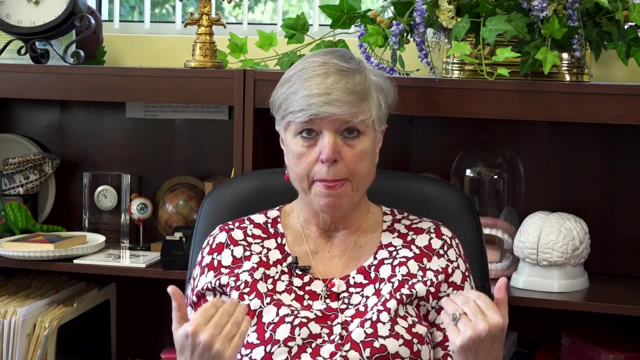 impact on the brain that if a child is reading something calling that number 16, they might be reading from the bottom up. They might even call that number 19 or 90. And so they're going to lose focus. So visual has a huge impact on the information going into the brain And there are 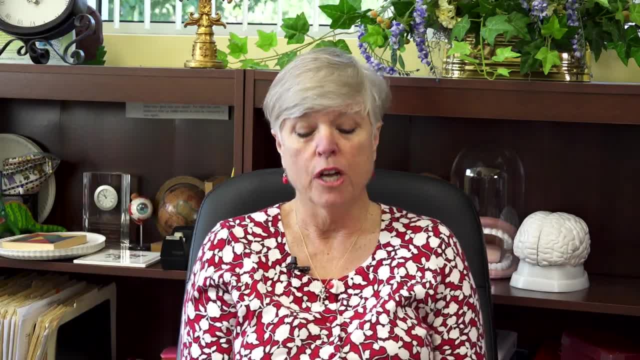 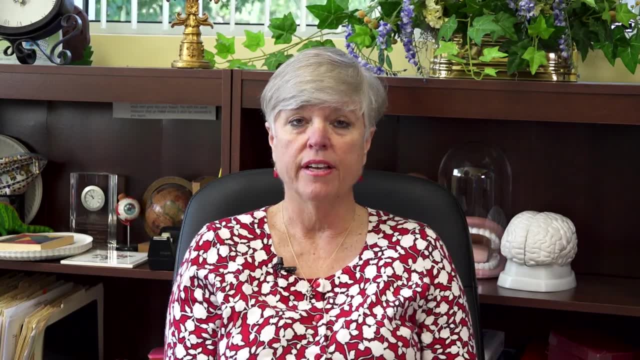 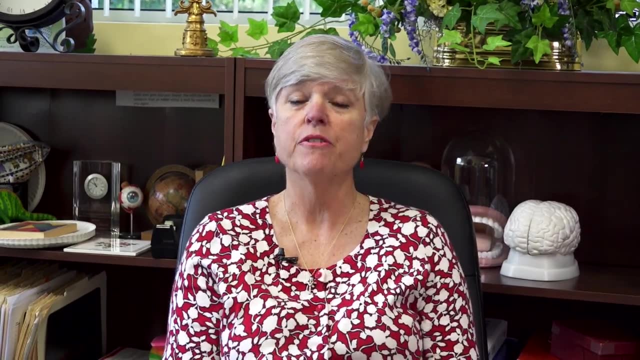 actually more cranial nerves that are coming from the eyes into the brain than that come from the ear to the brain. There's only one cranial nerve, number eight, that goes to the brain for auditory. There are over five that go from the eyes into the brain gathering information.